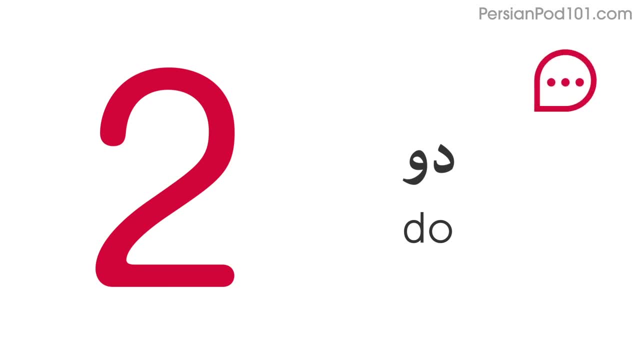 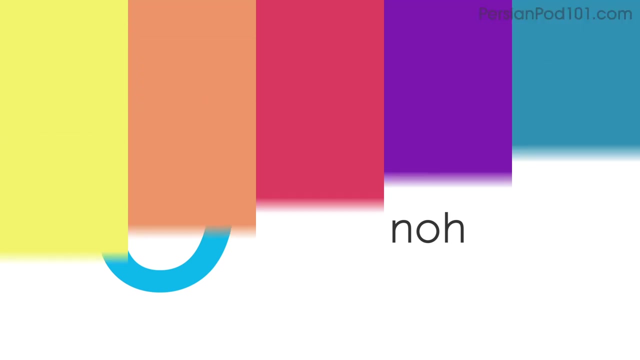 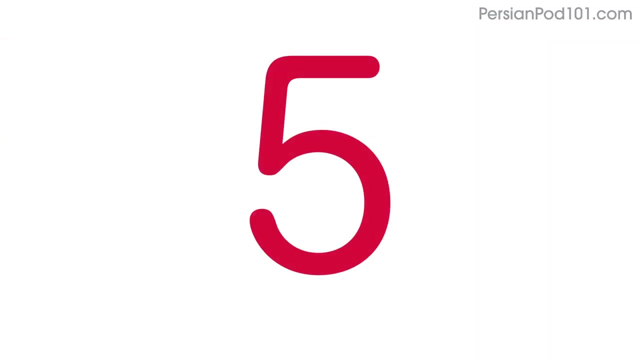 One, One, One, Two, Two, Two, Three, Three, Four, Four, Four, Four, Four, Four, Five, Five, Six, Six Half, Seven, Half Eight, Eight, Nine, Ten, Eleven, Twelve, Thirteen, Fourteen, Fifteen, Nineteen 얼마.